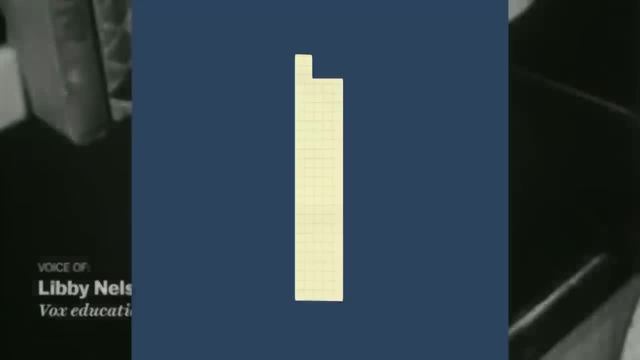 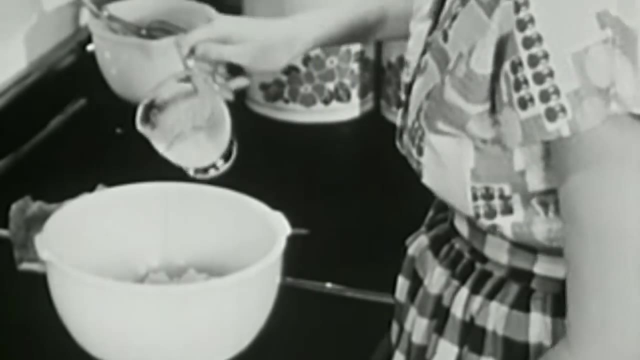 So math in some ways is like baking, and math used to be taught as a recipe, as a series of steps you do and then you get a result, And what you understand, if you're a cook or a baker, is that you add things in certain proportions for a reason, and that you know. 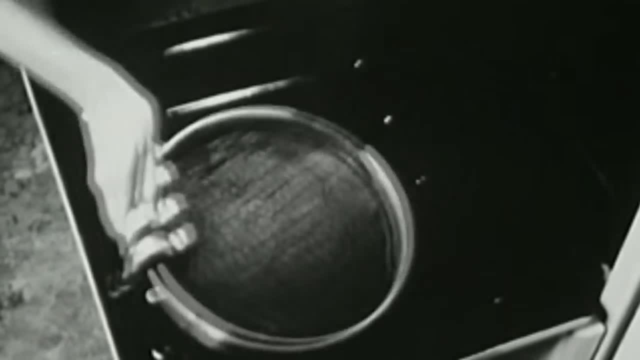 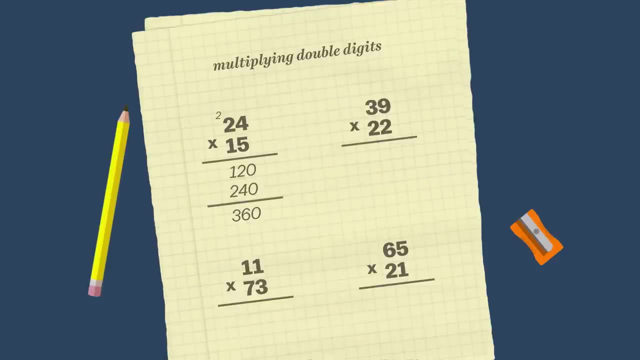 your cake has to have this percentage of fats to this percentage of flour in order to work. And what Common Core tries to do is to do the same thing with math, sort of developing what they call number sense. And number sense is understanding more or less why we do the. 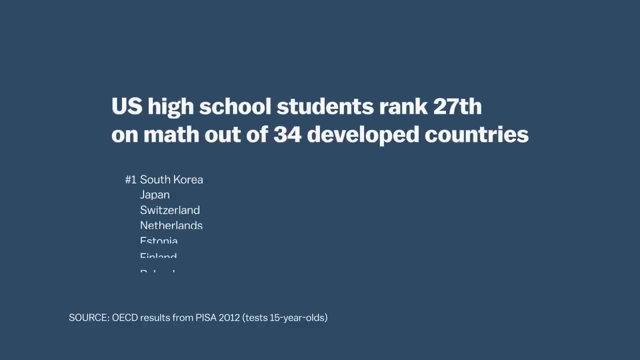 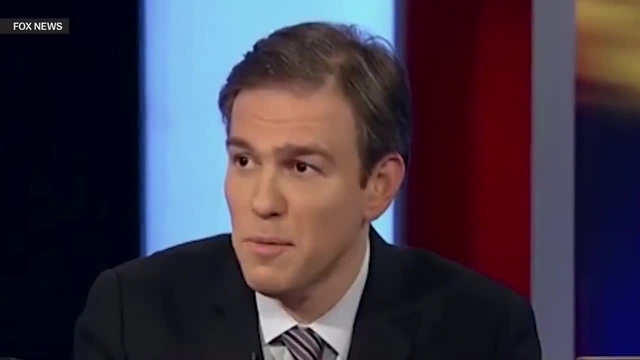 things we do. Common Core is taught in a way that most people over 20 don't recognize. We find ourselves tearing out our hair at the new math. It's the same thing I do when I get a check at a restaurant: draw a bunch of shapes and 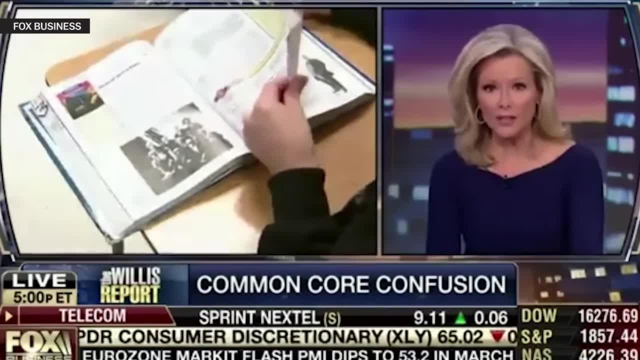 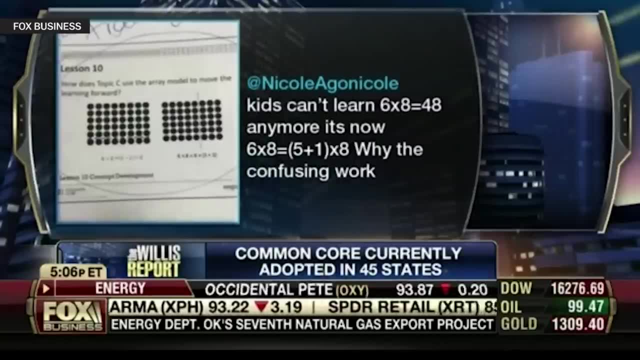 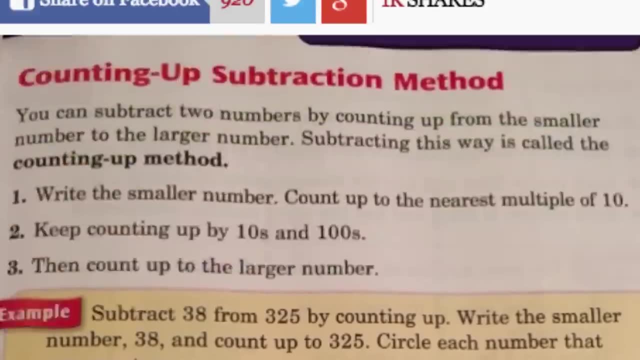 tell the waitress to find my error. Parents taking to Twitter posting unbelievably complicated homework assignments, These math problems circulate that just seem really nonsensical, which is really frustrating if you have a kid who has this simple problem. Yeah, That looks like it's being made way too complex for no reason. It's totally understandable. 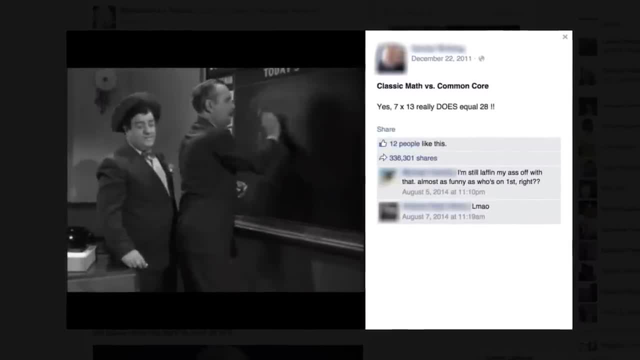 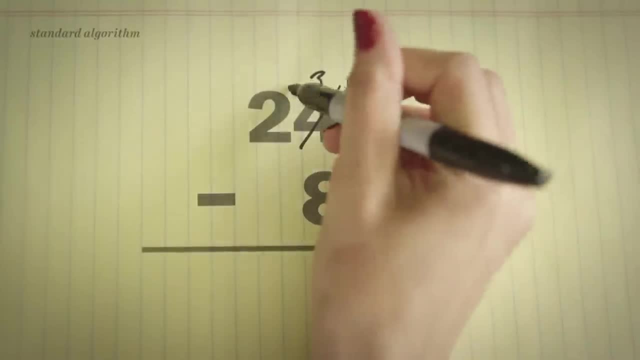 why people would say this recipe that I learned is the quick and easy way to do it. Why aren't they just teaching kids to do that? So, for example, we all learned to borrow when we subtracted, But this doesn't really show. 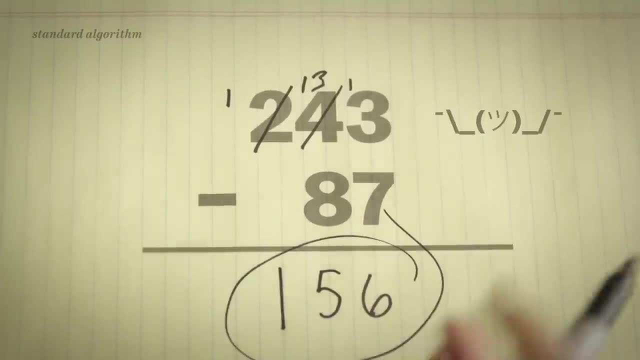 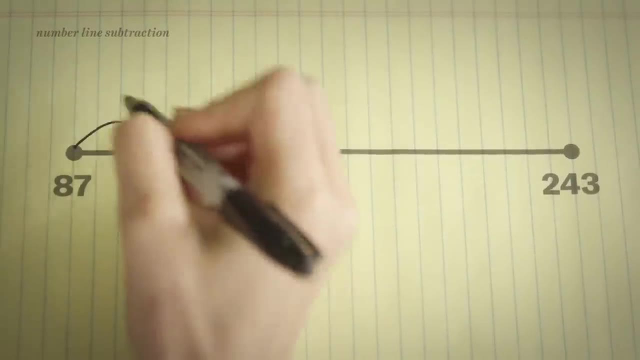 you what you're doing. It doesn't really show you what borrowing is, And so one of the ways the Common Core tries to explain this is with a number line, Because subtraction is really about finding the distance between two numbers. You start with the number line. 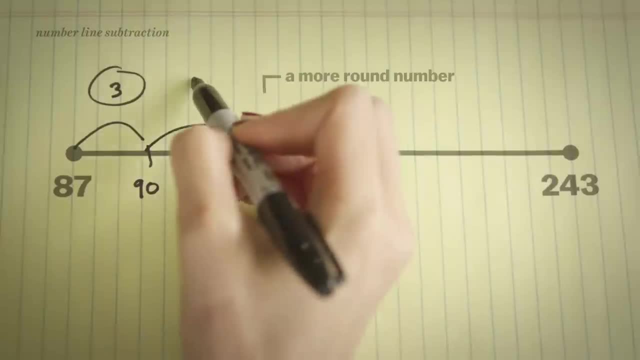 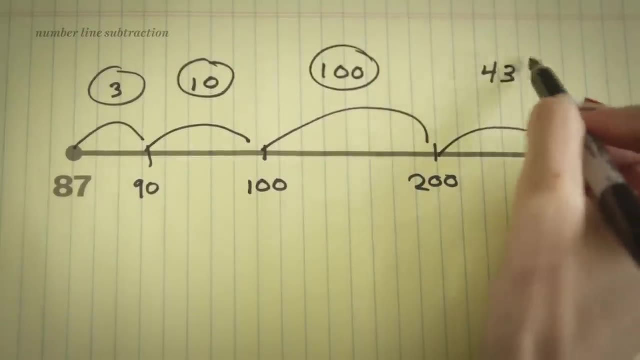 You start with the number you're subtracting And you take little hops up to a more round number. So you go 10 between 90 and 100. So you've sort of broken down this distance and you add these numbers together. There's another method called the counting up method, And this is also for subtraction. 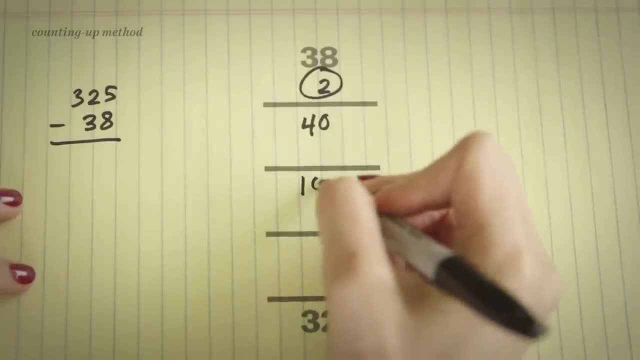 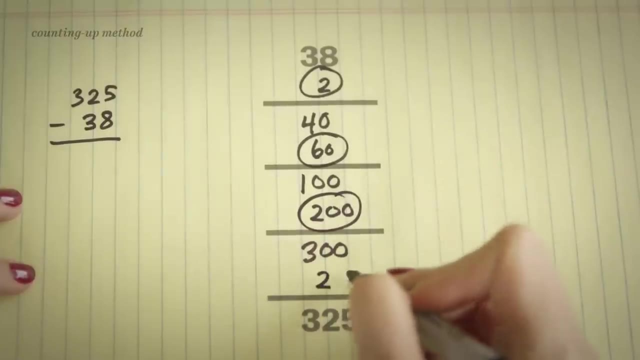 Count up from 38 to 40. Then from 40, you want to go up to the next big round number, which is 100. Then you need to go from 100 to 300. And then from 300 to 325.. So that's.